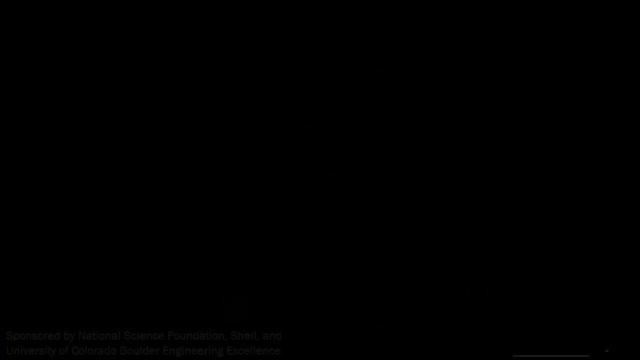 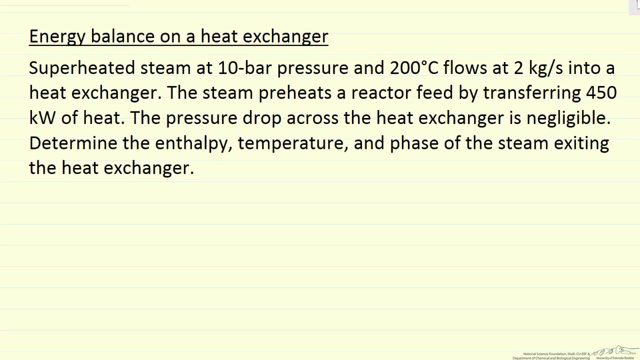 This problem. we're asked to do an energy balance on heat exchanger. We're given the feed which is superheated steam and we tell how much energy is removed from that steam to heat some reactor feed. We want to know what's the outlet temperature of the steam, what? 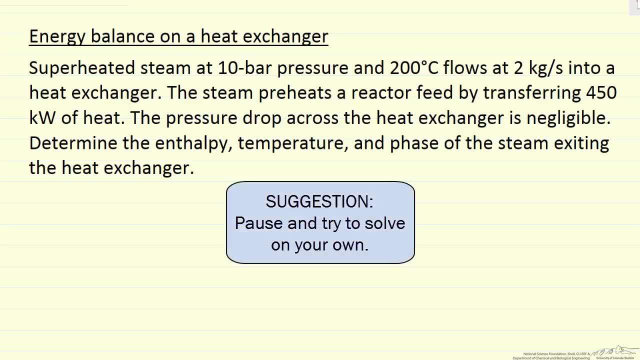 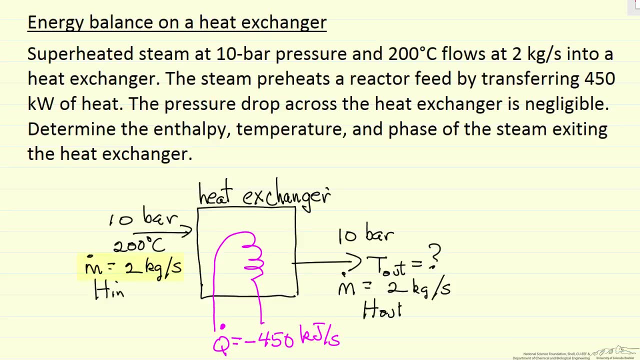 phase is it in, and then what's the enthalpy? So the first thing I'm going to do is draw a diagram so we can input the information we already know about the system. So here we're showing the mass flow rate in m dot. 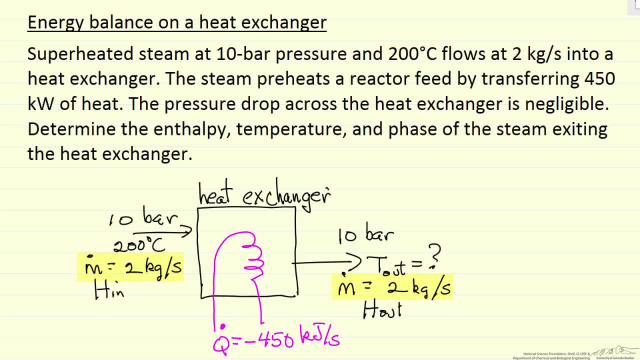 That's a constant, so the same mass is leaving. We don't know the outlet temperature and the heat removed is negative. That's taken as my system to steam. so I'm removing 450 kilojoules per second, which corresponds to: 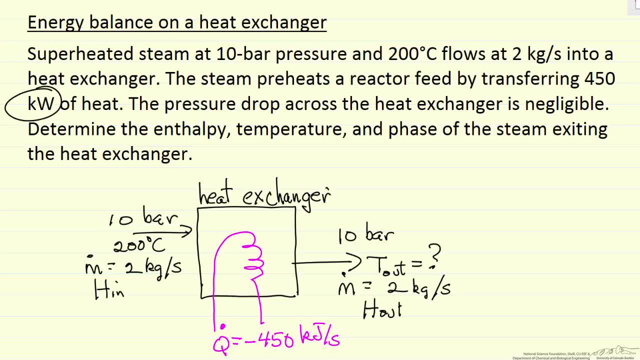 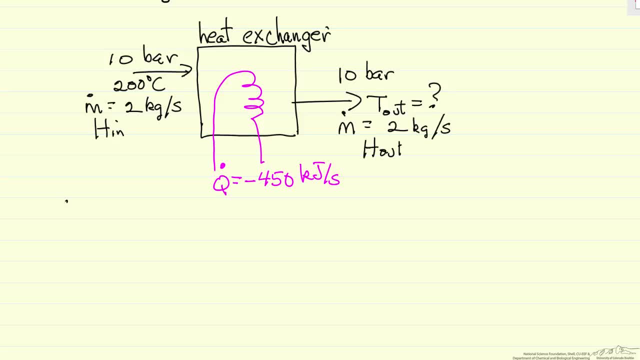 450 kilowatts. So what I want to do is an energy balance. It's a steady state system and so the energy balance is going to be steady state. We have energy flowing into the system, an inlet stream, Same mass flow rate. out Enthalpy is going to be different, And then we have a rate of 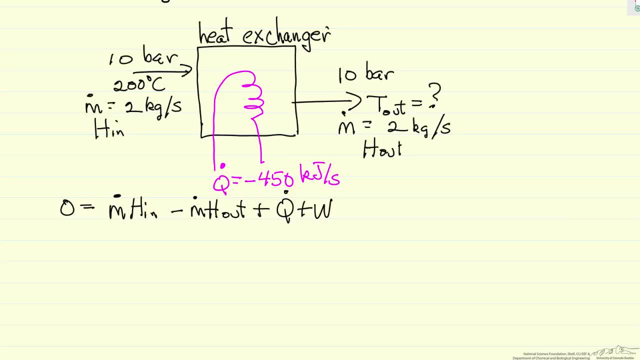 heat removal. Of course, in general we would have work, but There's no work in this system. The first thing we're going to do is look up the inlet enthalpy using steam tables. So 200 degrees C, 10 bar goes to superheated steam tables and we know it's a superheated. 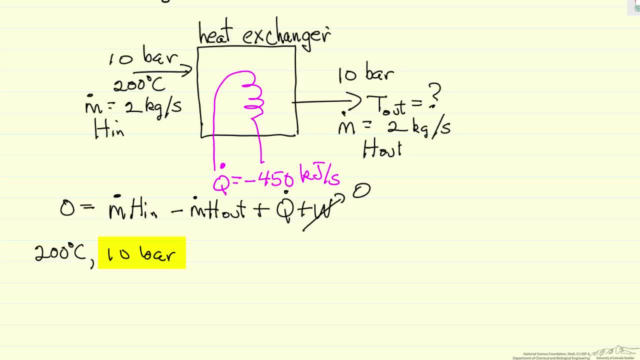 one, because this pressure is less than saturation pressure and because the problem statement points it out. And so the enthalpy. I can just read directly, The enthalpy coming in: 28,, 28 kilojoules per kilogram. 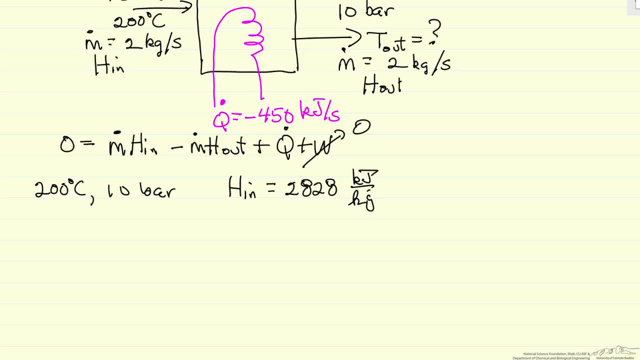 I can solve this equation for the enthalpy out. So let me first rearrange the equation, the energy balance. So I rearrange the energy balance by taking these two terms, the other side of the equation, And then I substitute in the values for Q dot and M dot.